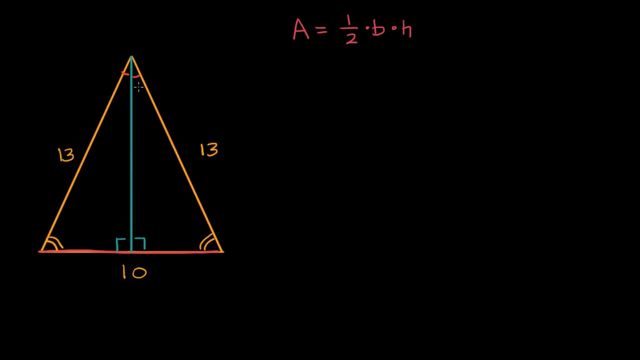 notice that they both have a side 13,. they both have a side, whatever this length blue is, and so, and then they're both going to have a side length. that's half of this 10. So this is going to be five and this is going to be five. 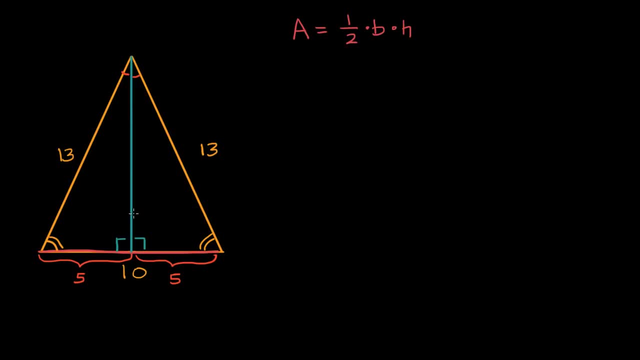 How was I able to deduce that? You might just say: oh, that feels intuitively right. I was a little bit more rigorous here, where I said: oh, if these are two congruent triangles, then we're going to split this 10 in half. 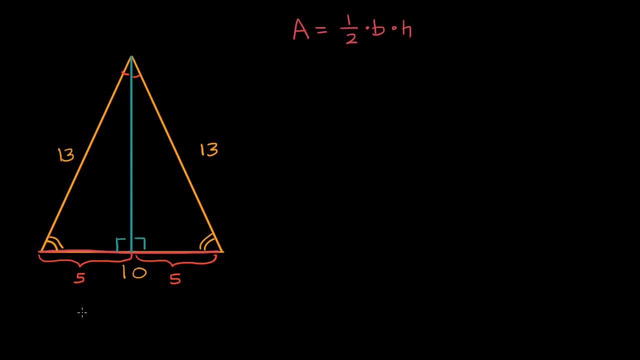 because this is going to be equal to that and they add up to 10.. All right, now we can use the Pythagorean theorem to figure out the length of this blue side, or the height. If we call this h, the Pythagorean theorem tells us: 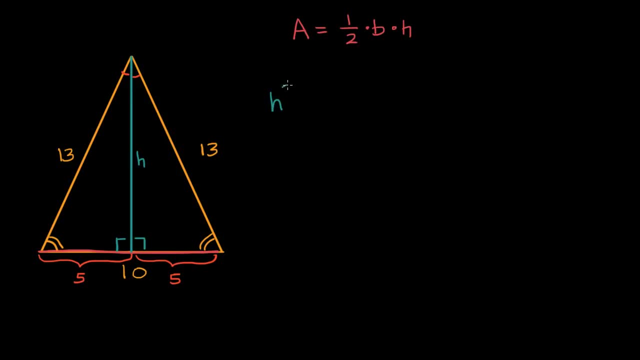 that h squared plus five squared is equal to 13 squared. h squared plus five squared plus five squared is going to be equal to 13 squared. It's going to be equal to our longest side, our hypotenuse squared. and so let's see. 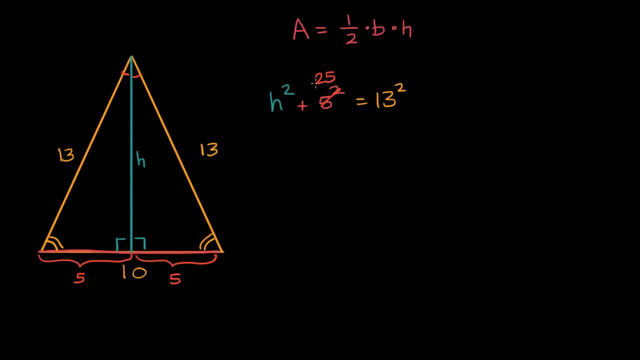 Five squared is 25.. 13 squared is 169.. We can subtract 25 from both sides to isolate the h squared. so let's do that, and what are we left with? We are left with h squared. h squared is equal to these canceled out. 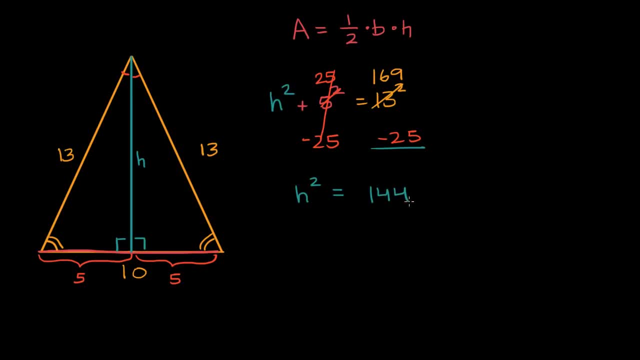 169 minus 25 is 144.. Now, if you're doing it purely mathematically, you say: oh, h could be plus or minus 12, but we're dealing with the distance, so we'll focus on the positive. 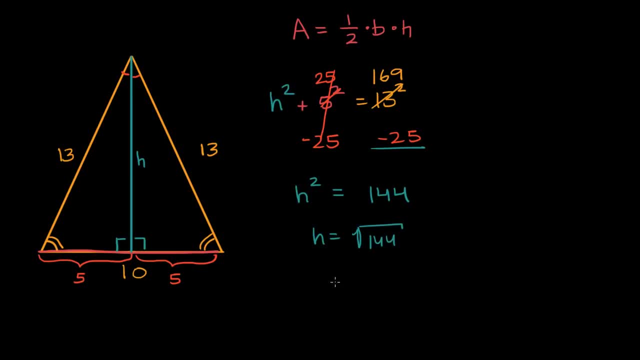 so h is going to be equal to the principal root of 144, so h is equal to 12.. Now we aren't done. Remember, they don't want us to just figure out the height here, They want us to figure out the area. 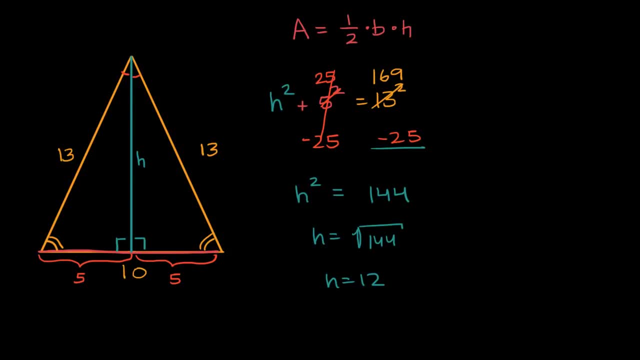 Area is 1 1⁄2 base times height. Well, we already figured out that our base is this: 10. right over here Let me do this in another color. So our base is that distance, which is 10, and now we know our height. 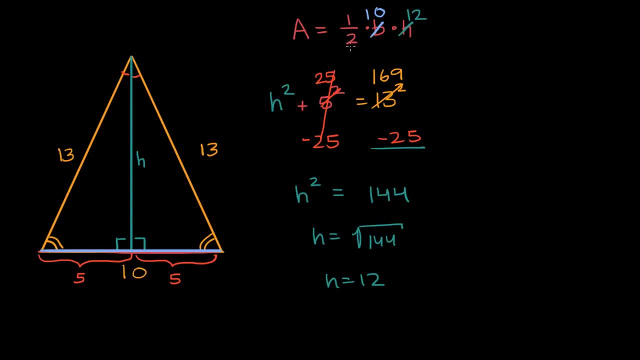 Our height is 12.. So now we just have to compute 1 1⁄2 times 10 times 12.. Well, that's just going to be equal to 1 1⁄2 times 10 is 5 times 12 is 60, 60 square units. 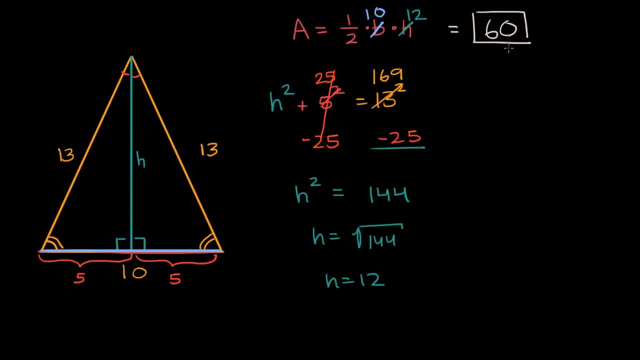 whatever our units happen to be, That is our area.